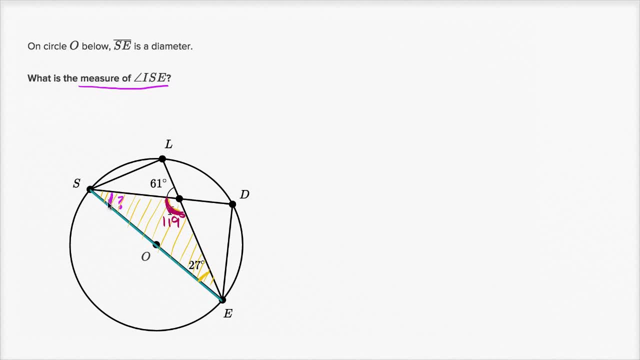 And so this angle that we're trying to figure out, this angle plus the 119 degrees, plus the 27 degrees, is going to be equal to 180 degrees, Or we could say that this angle is going to be 180 minus 119, minus 27,. 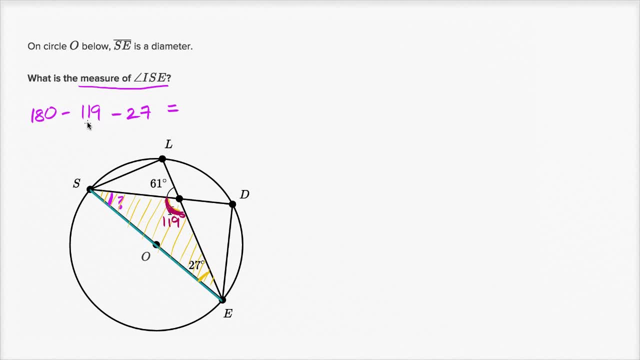 which is going to be equal to. So let's see: 180 minus 119 is 61, and then 61 minus 27 is going to be 34.. So there you have it. Measure of angle: ISE is 34 degrees. 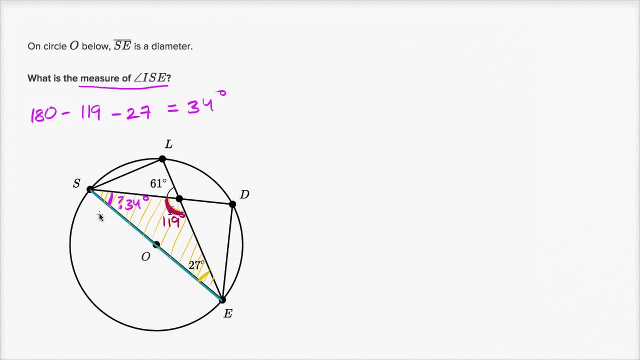 Now I mentioned that there is multiple ways that we could figure this out. Let me do it one more way. So let me unwind everything that I just wrote. We already figured out the answer, but I want to show you that there's multiple ways. 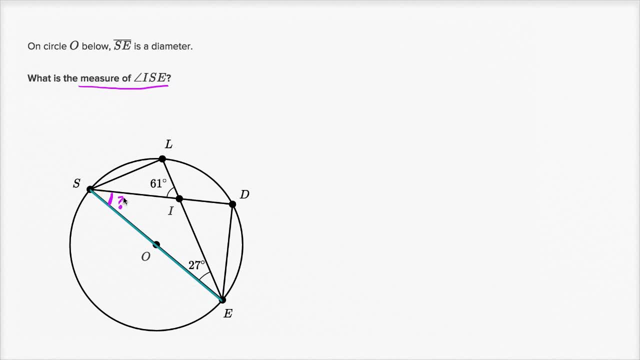 that we can tackle this. So ISE is still the thing that we want to figure out. Another way that we could approach it is: well, we know we have some angles, inscribed angles, on this circle, and we know that if an inscribed angle 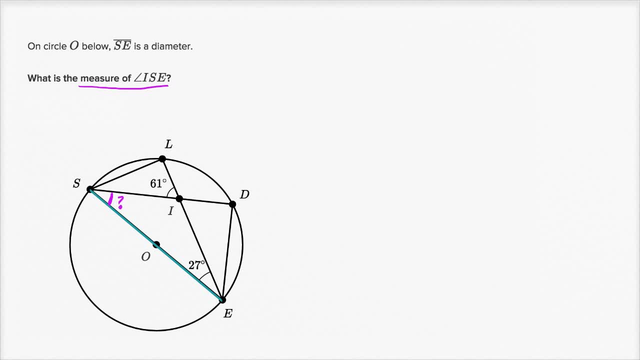 intercepts the diameter, then it's going to be a right angle. It's going to be a 90-degree angle. So this angle right over here is a 90-degree angle and we can use that information to figure out and this angle 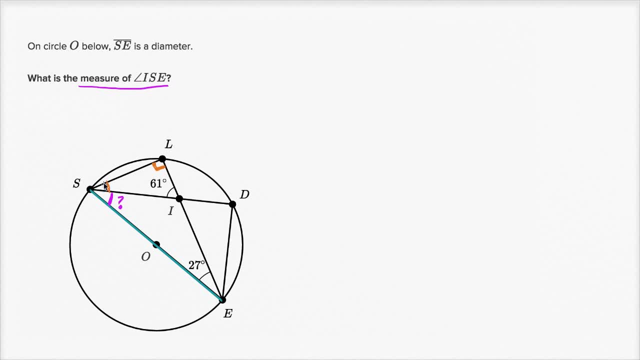 and we could also use that information if we look at a different. so if we look at this triangle, we could use 90 plus 61 plus this angle is going to be equal to 180 degrees. So this angle right over here, another way to think about it. 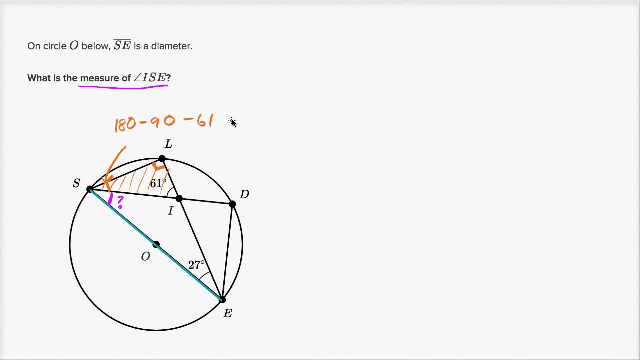 it's going to be 180 minus 90 minus 61, which is equal to 180 minus 90, is 90 minus 61 is 29 degrees. So this one right over here is 29 degrees. 29 degrees. And then we could look at this larger triangle. 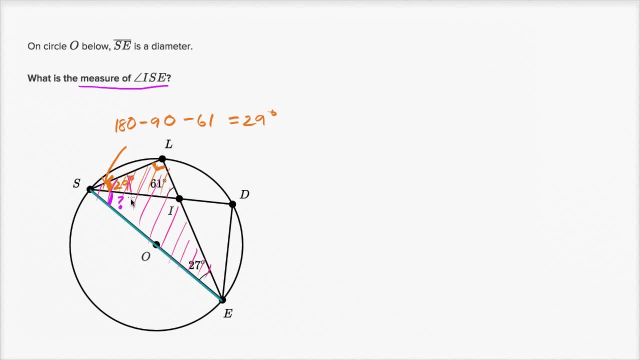 We could look at this larger triangle right over here to figure out this entire angle. to figure out this entire angle, If we know this entire angle, you subtract 29,, then you figure out angle ISE, And so this large or what I've depicted is this kind of.